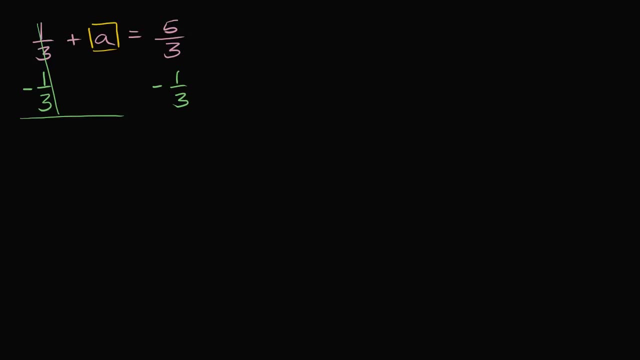 that's the whole reason why I subtracted 1- 3rd was to get rid of the 1 3rd and I am left with a is equal to 5 3rds minus 1 3rd. 5 3rds minus 1 3rd minus 1 3rd. 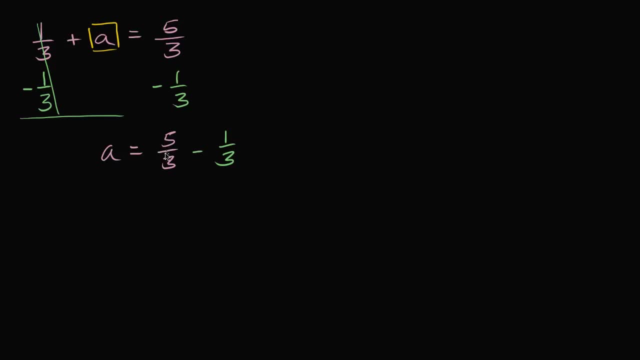 And what is that going to be equal to? I have 5 of something. in this case I have 5 3rds and I'm going to subtract 1 3rd, So I'm going to be left with 4 3rds. 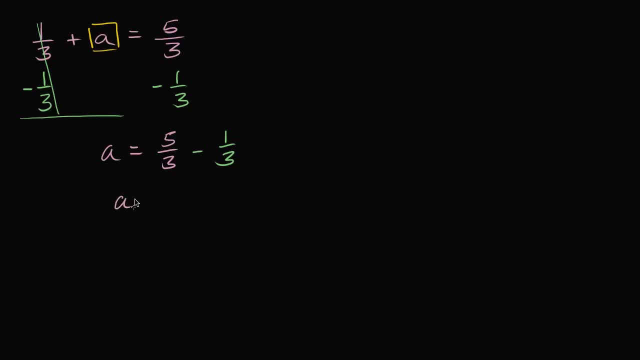 So I could write a. a is equal to 4 3rds And you could check to make sure that works: 1 3rd plus 4 3rds is indeed equal to 5 3rds. Let's do another one of these. 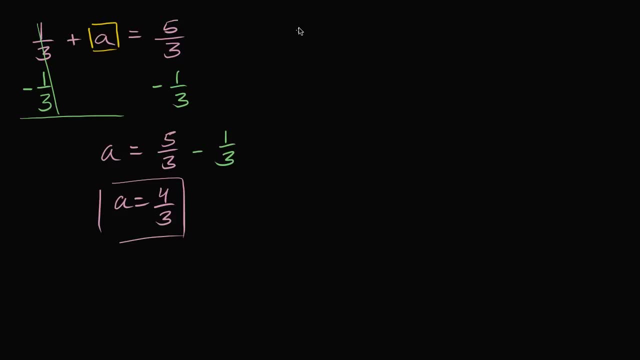 So let's say that we have the equation: k minus 8 is equal to 11.8.. So once again I want to solve for k. I want to have just a k on the left-hand side. I don't want this subtracting this 8 right over here. 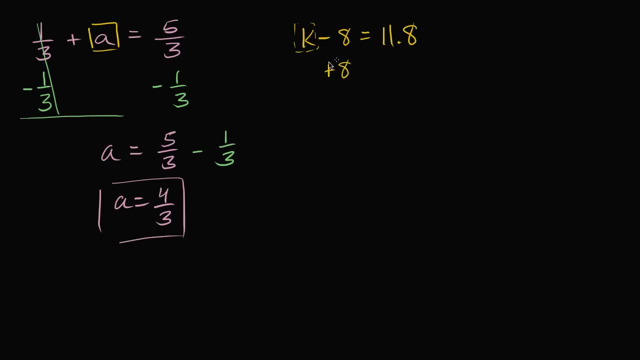 So, in order to get rid of this 8, let's add 8 on the left-hand side, And, of course, if I do it on the left-hand side, I have to do it on the right-hand side as well. So we're going to add 8 to both sides. 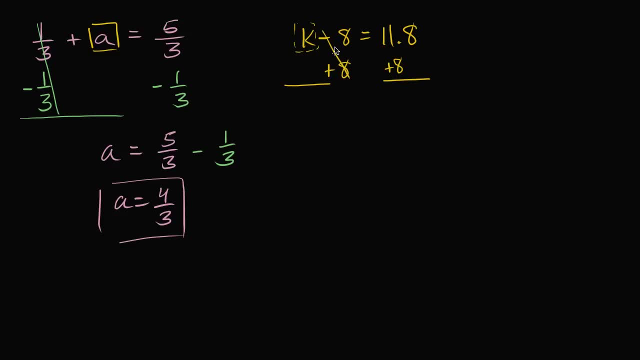 The left-hand side, you are subtracting 8, and then you're adding 8. That's just going to cancel out and you're just going to be left with k And, on the right-hand side, 11.8 plus 8.. 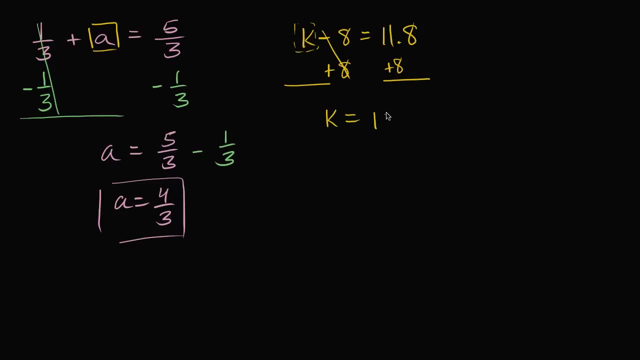 Well, 11 plus 8 is 19,. so it's going to be 19.8.. And we're done. And once again, what's neat about equations: you can always check to see if you got the right answer. 19.8 minus 8 is 11.8.. 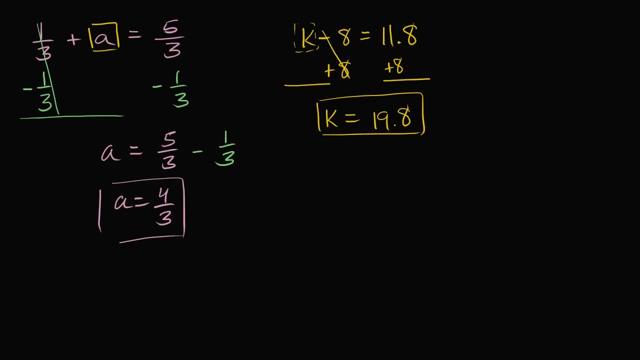 Let's do another one. This is too much fun, All right. So let's say that I had 5 13ths is equal to t minus 6 13ths. All right, this is interesting because now I have my variable on the right-hand side. 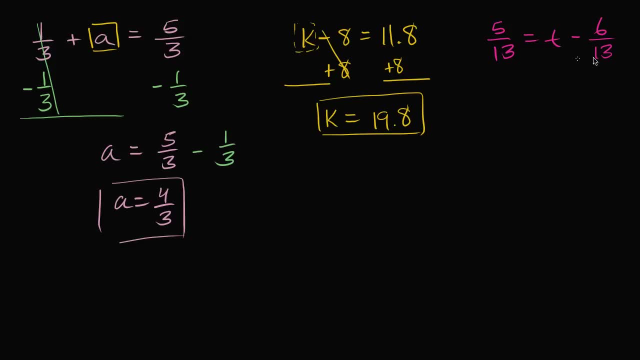 But let's just leave it there. Let's just see if we can solve for t by getting rid of everything else on the right-hand side And, like we've done in the past, if I want to, I'm subtracting 6 over 13,.